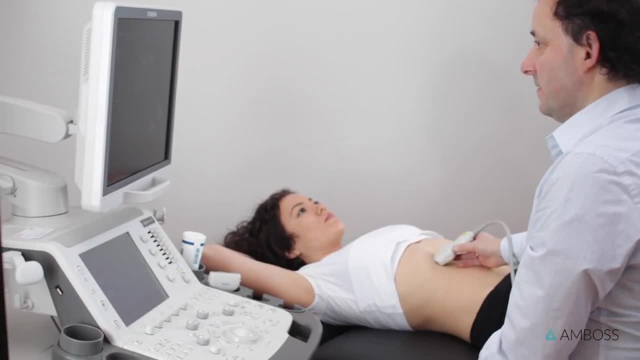 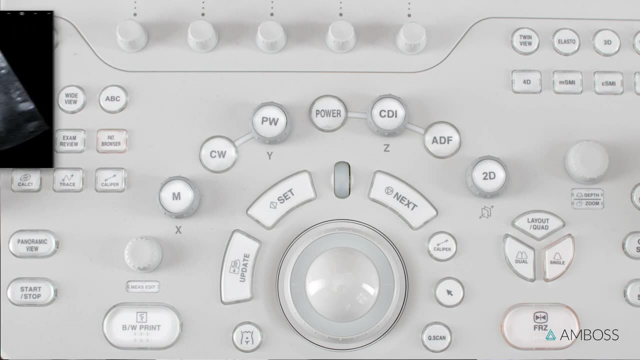 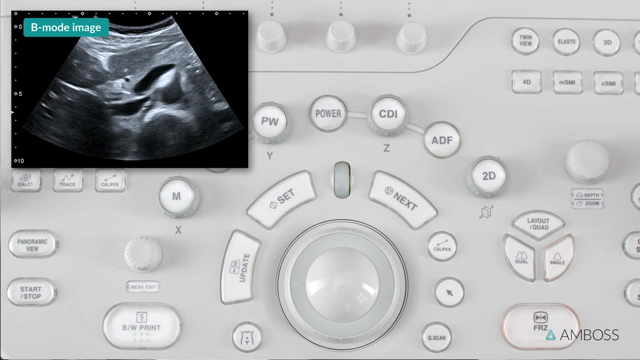 To generate reliable images and interpret them correctly, you need to understand the basic functions of the ultrasound machine and how to set them up. Most important is learning how to set up the B-mode image which you'll use in almost all scans. On most modern machines, the basic ultrasound functions are controlled using the knobs and buttons of a console. 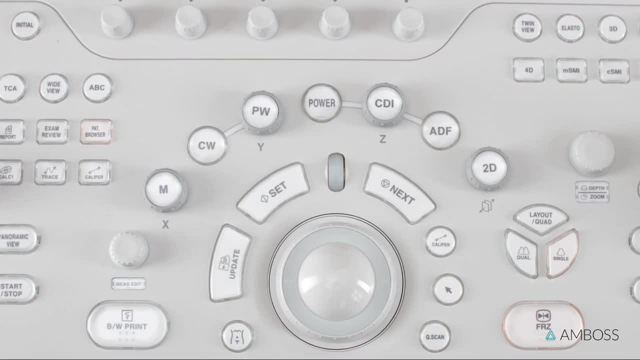 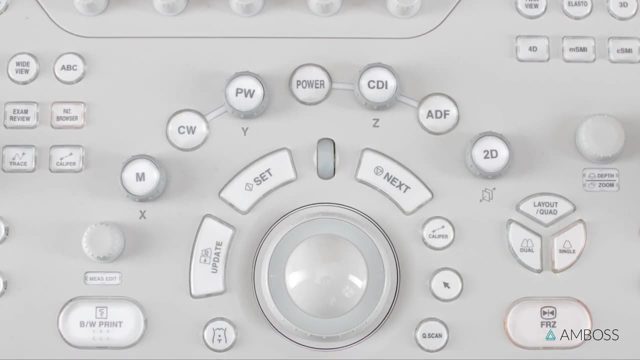 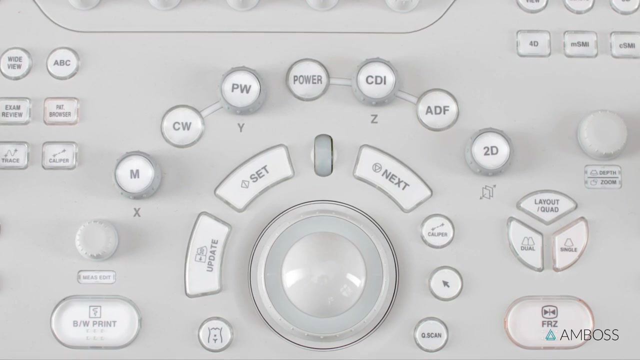 The position and appearance of the controls vary, so you should familiarize yourself with the new machine before getting started. However, most of the basic functions can be found relatively easily on all machines. More complex or manufacturer-specific functions like 3D ultrasound are not covered in this video. 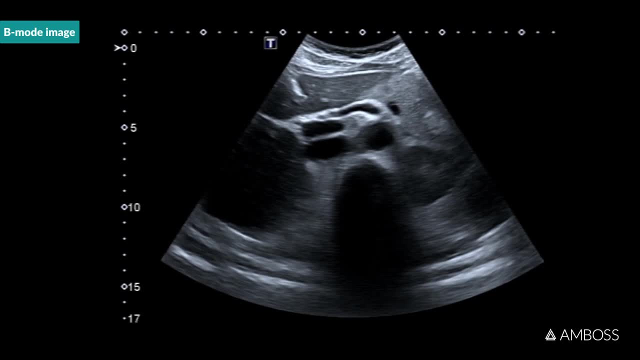 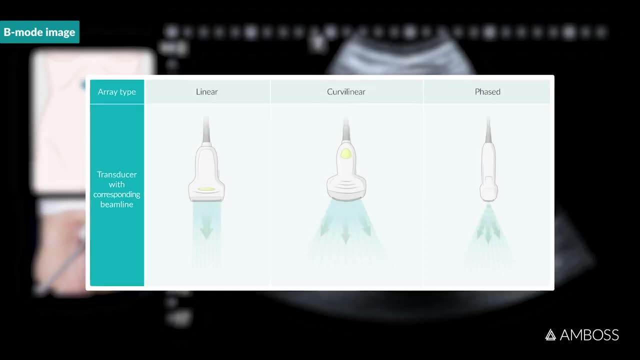 Setting up the Ultrasound Machine- The B-Mode Image At the start of every scan. the B-Mode Image should be optimized to best display the area of interest. In this example, we're using a curvilinear probe to show a transverse scan of the upper abdomen. 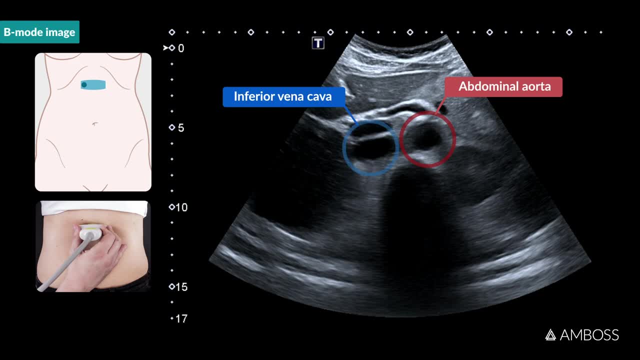 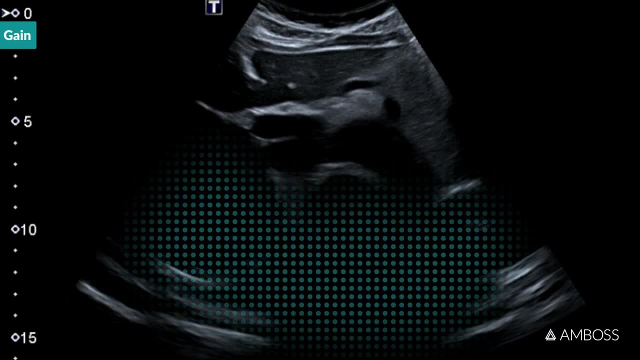 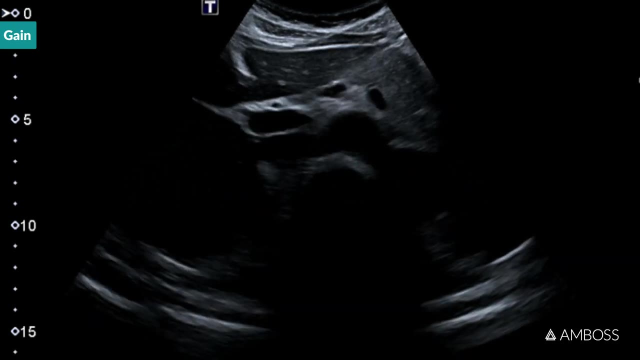 We'll now adjust the image to show the aorta and inferior vena cava as clearly as possible. 220 00R Gain. At the moment there are a lot of dark areas in the image that are effectively information-free. We can make these clearer by increasing the amplification of the reflected ultrasound signal in the image, the so-called gain. 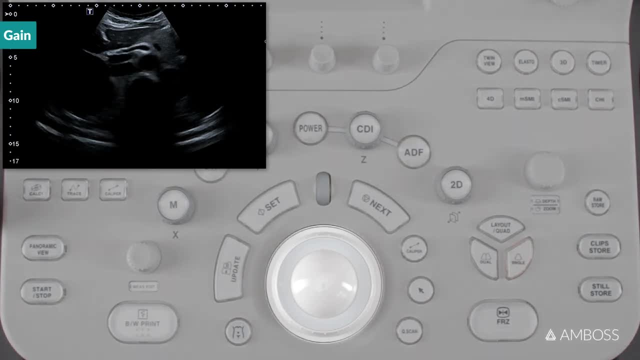 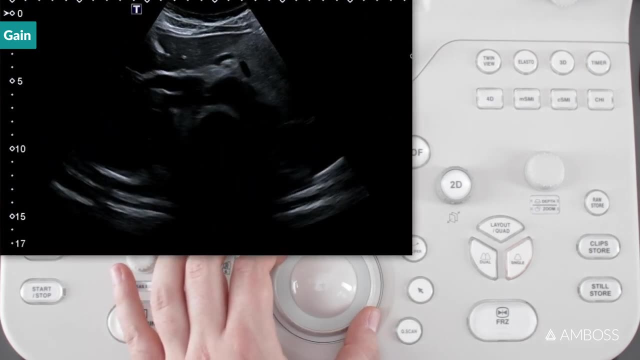 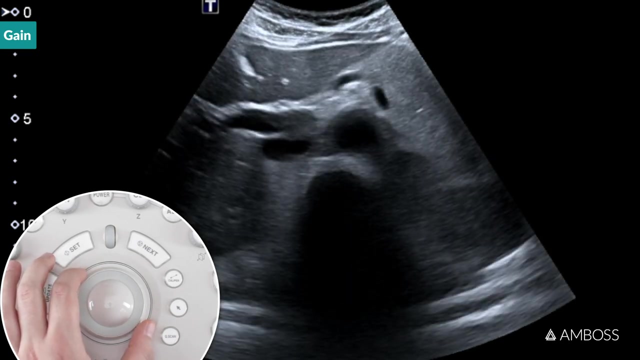 On this machine, gain is controlled using a rotary control in the middle of the console, similar to a volume knob. Increasing gain makes the entire image brighter. If gain was previously set too low, as shown here, increasing it can make it easier to distinguish structures of interest. 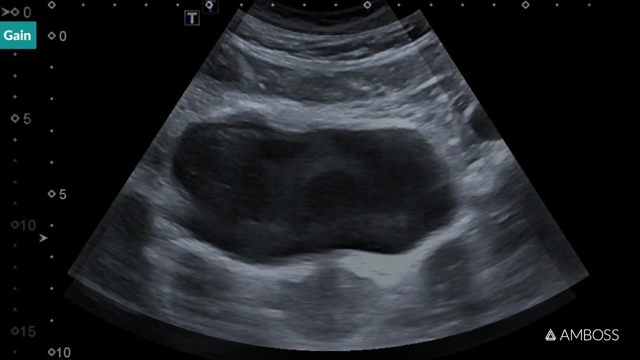 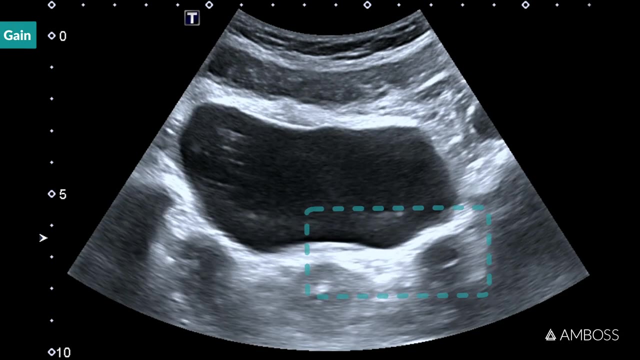 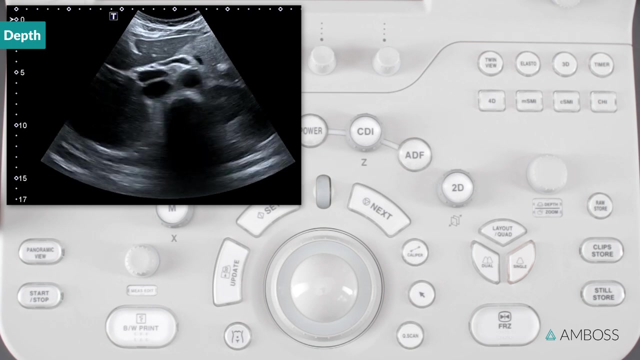 But the gain should not be set too high either, because this overgain will make the image too bright, amplify noise and reduce your ability to differentiate tissues Depth. To best assess your structures of interest, they should be displayed as largely as possible and centered on the screen. 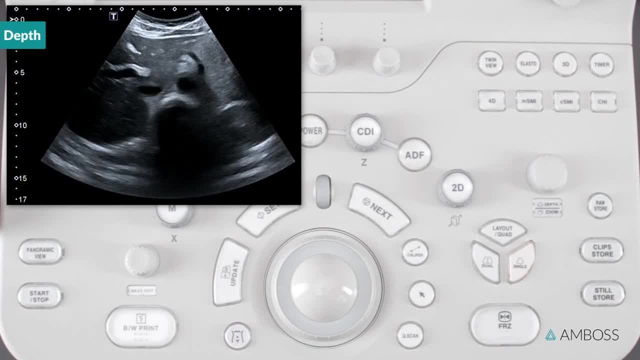 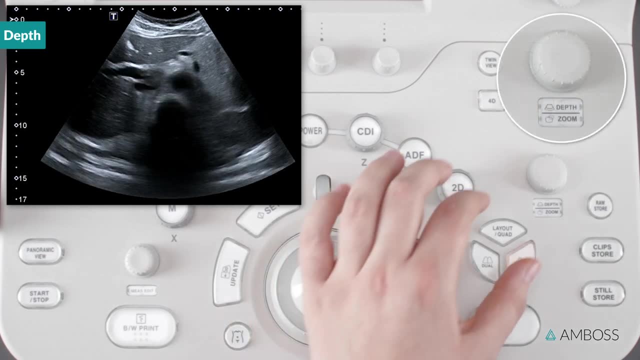 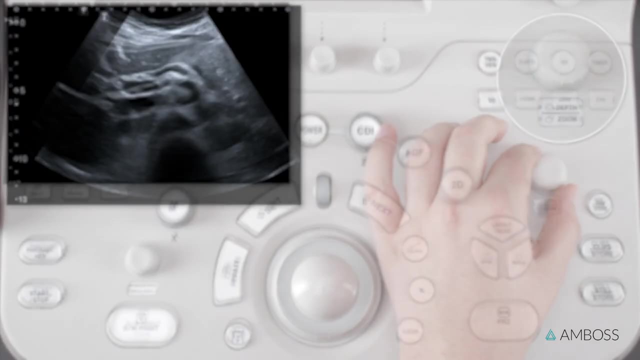 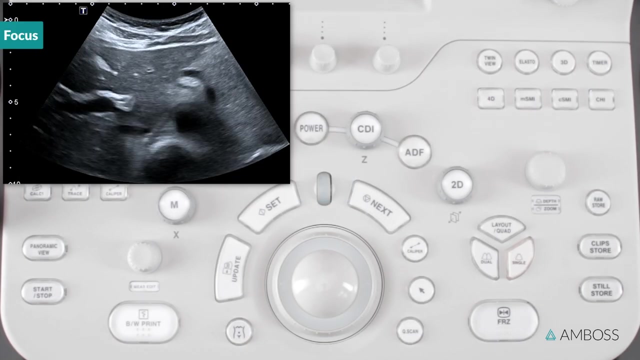 We do this by adjusting the penetration depth of the ultrasound signal to the minimum required to still allow all structures of interest to be visualized. On the machine shown here, this is done using the rotary control labeled Depth, Zoom, Focus. Image resolution can be selectively increased in the area of interest by adjusting the focal zone. 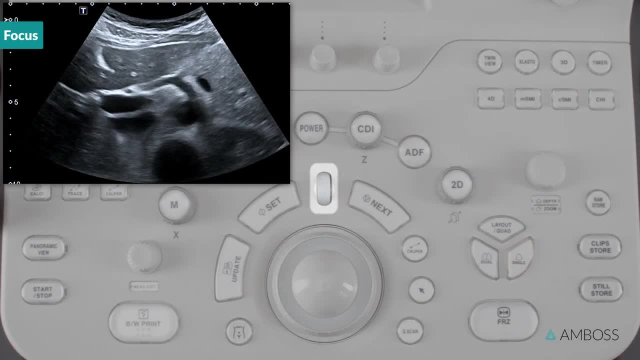 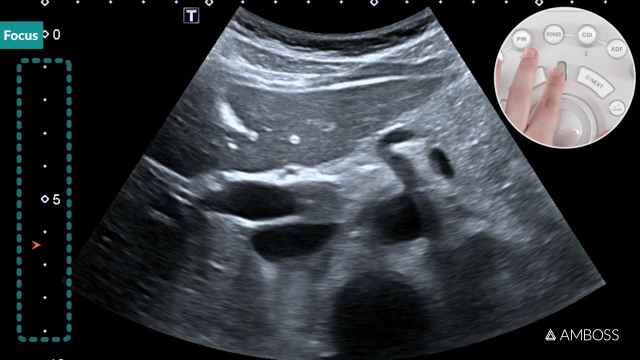 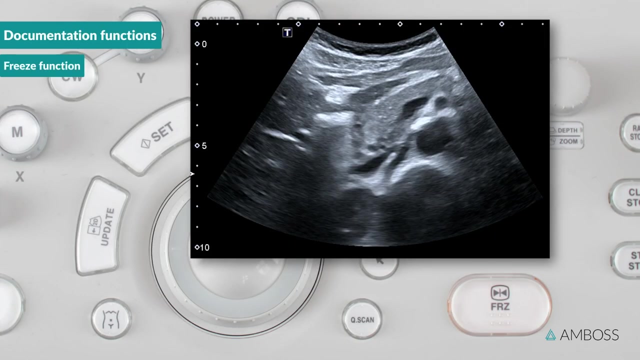 On the machine shown here, this is done using another rotary control. The changing focal zone is shown by a moving arrow on the left side of the image. Documentation Functioning- Documentation Functioning- Documentation Functioning. When performing a scan, it can be very helpful to freeze the image at a specific point in time. 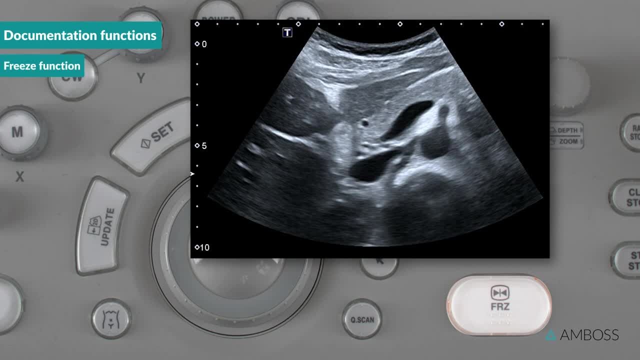 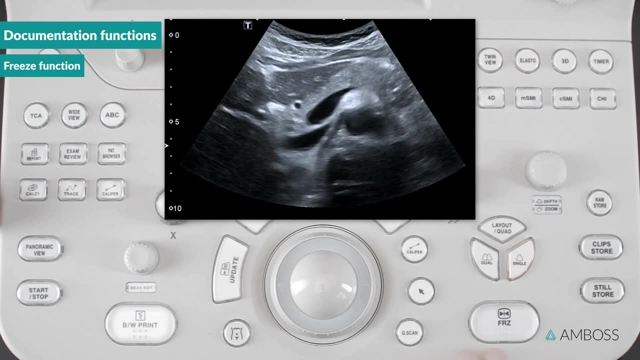 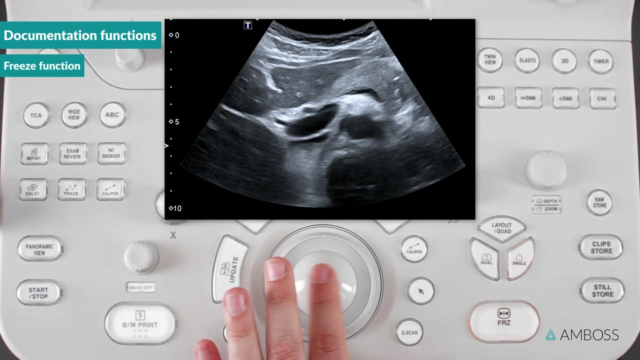 You can do this using the Freeze function. On the machine shown here, the Freeze button is labeled FRZ and is located on the lower right of the console. Pressing the button freezes the current image. Once you've pressed Freeze, most machines allow you to scroll back through the most recent frames to select the best one. 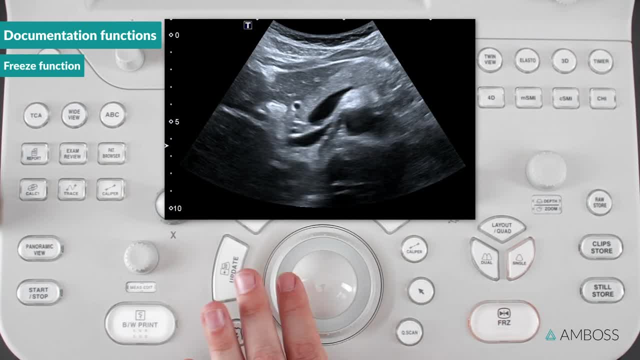 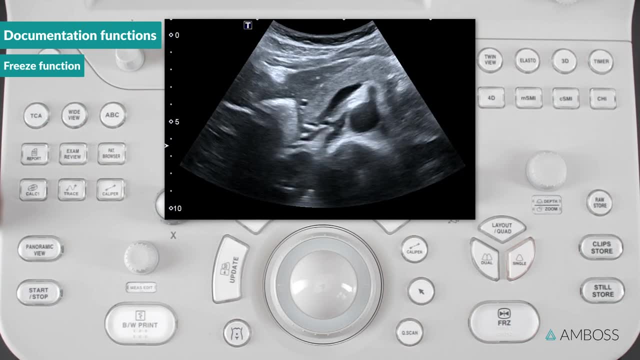 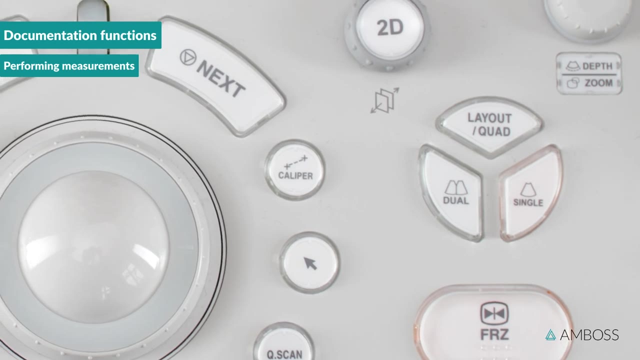 On the machine shown here. you can scroll using the trackball in the center of the console and pressing the Freeze button again returns to the real-time image. When performing measurements, you can also perform measurements. Once you've frozen the image, you can also perform measurements. 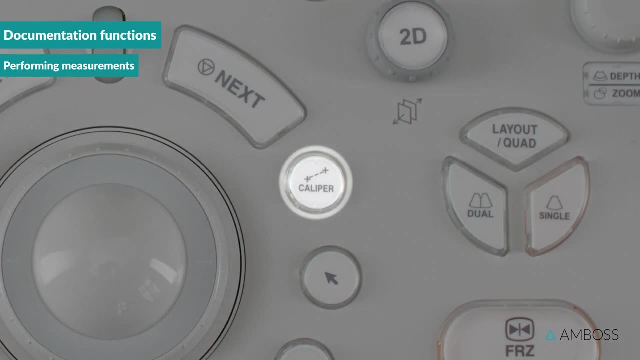 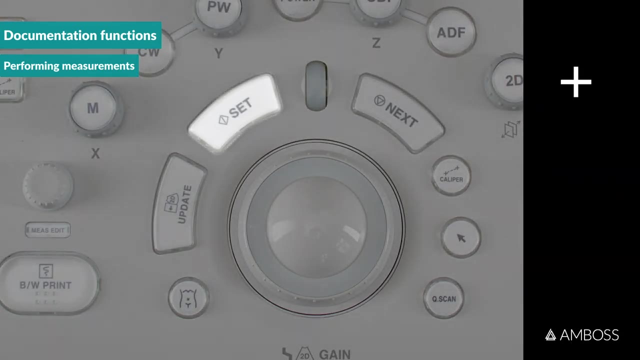 On the machine shown here, this function is activated by pressing the Caliper button. Next, confirm the starting point of your measurement by pressing the Set button. Then press the Caliper button. Next, confirm the starting point of your measurement by pressing the Set button. 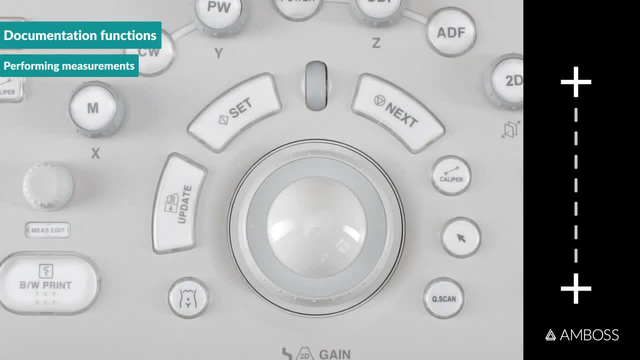 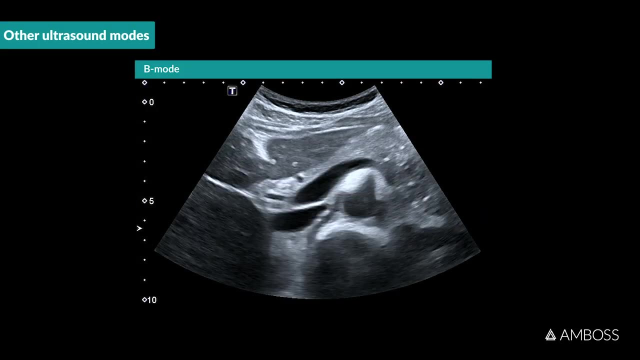 Then use the trackball to navigate to the end point. Press Set again to confirm and display the result. Pressing the Next button allows you to take another measurement. Other ultrasound modes In addition to B-mode, there are other scanning modes that provide further information. 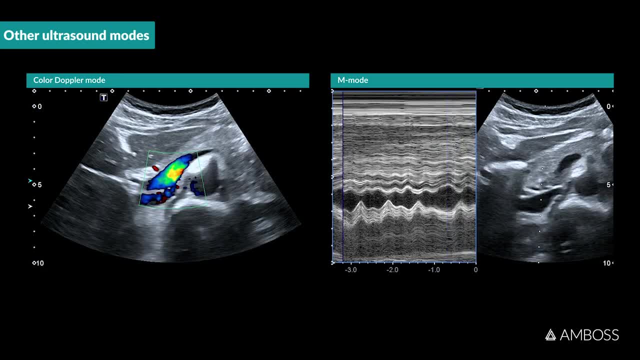 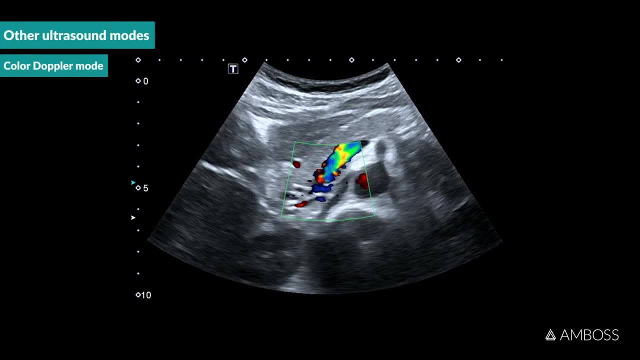 We'll look at two of these next: Color Doppler mode and M-mode Color Doppler mode. Color Doppler mode is used to look for a scan. Color Doppler mode is used to look for a flame. Color Doppler mode is used to look for the presence of flow, usually the movement of blood in arteries and veins. 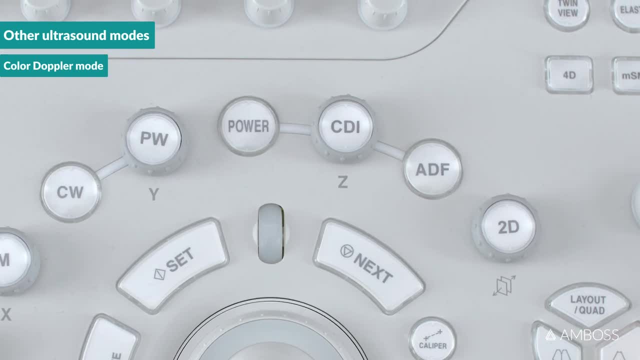 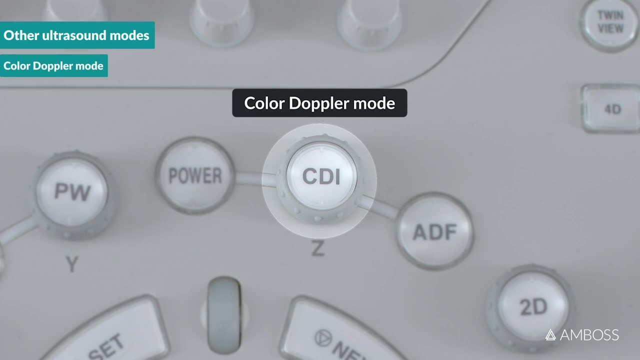 On the machine shown here. this function is activated and deactivated by pressing the CDI button, which stands for color-doppler imaging. Other manufacturers label this differently. Other manufacturers label this differently, For example, C for color or CF for color flow. 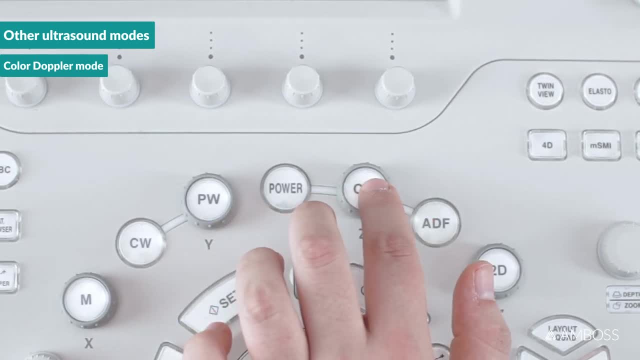